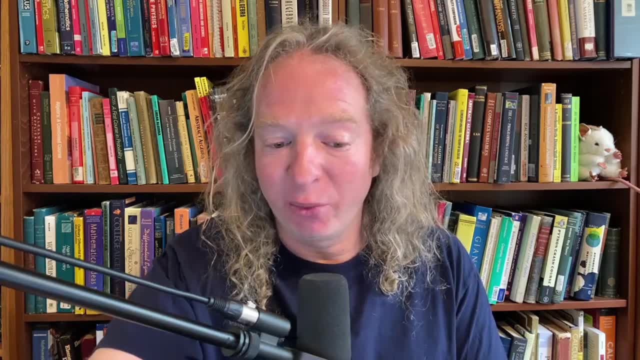 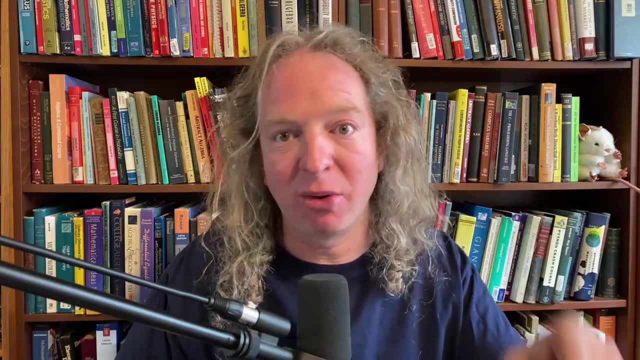 partial differential equations, So that's actually a really good question. So, personally, let me just say that I've taken one class on partial differential equations, So I have- that's my experience- right- One undergraduate class at the undergraduate level where we 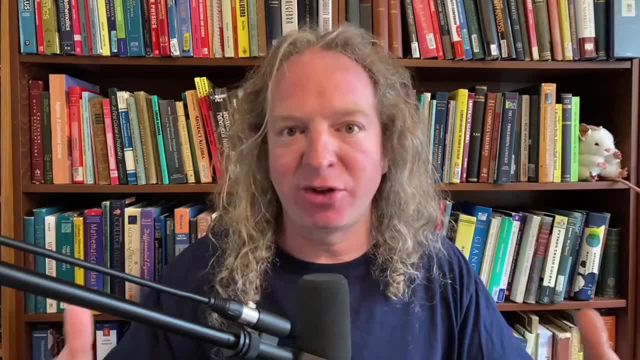 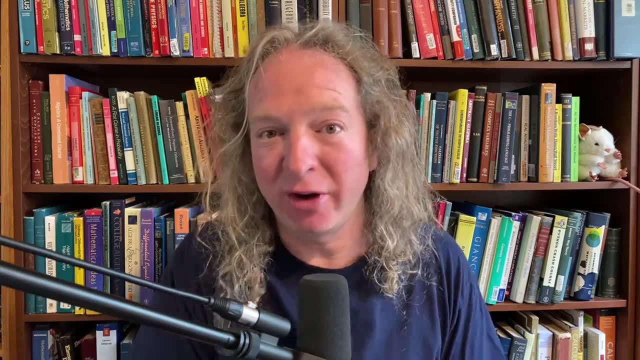 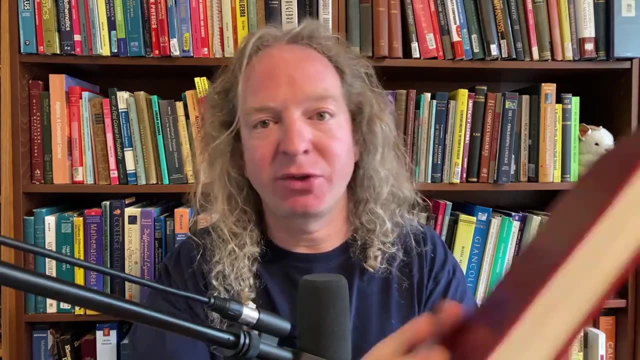 studied most of the core basic techniques to solve PDEs And I found that the problems themselves were very, very long and they took a very long time to solve. The book I used was the book by Strauss which I have right here called Partial Differential. 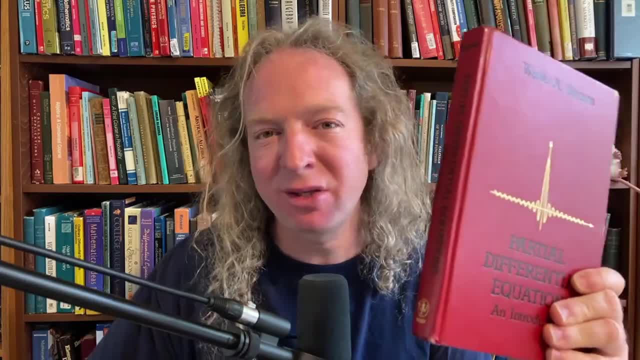 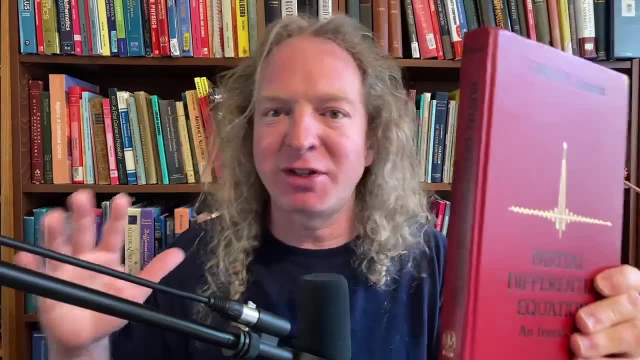 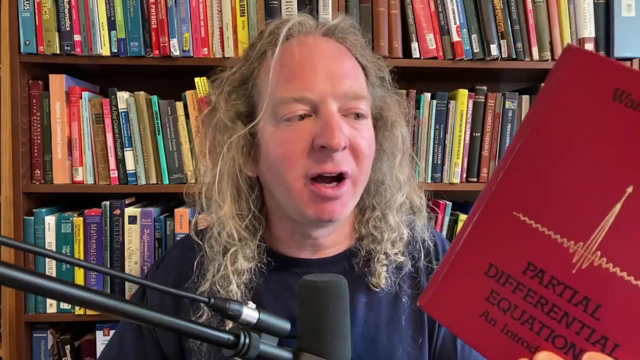 Equations by Walter Strauss And honestly, I think this is an okay book. I'm not going to tell you that it's a great book. I think it's an okay book and it's pretty good. That's as far as I'll go, And my reason for not saying it's a great book is twofold One: I found that the 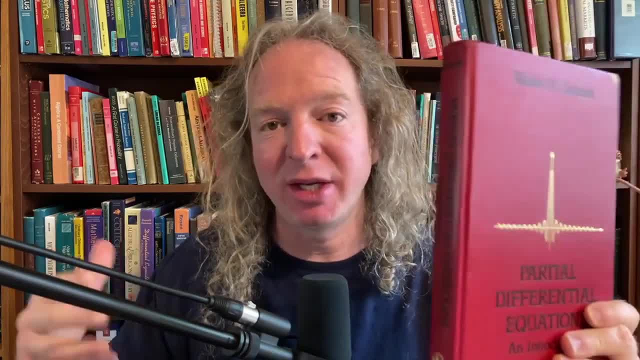 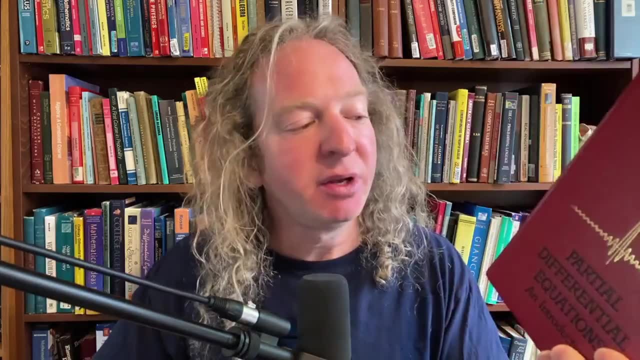 explanation of the problem itself was very, very long And I found that the explanation of the were a bit terse at the time when I was taking the class. Reading it now it reads a little bit better. Two: there are some typos in the solutions, just a few. So still worth picking up, still worth. 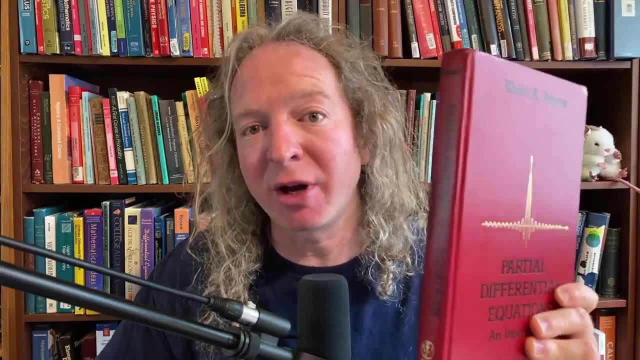 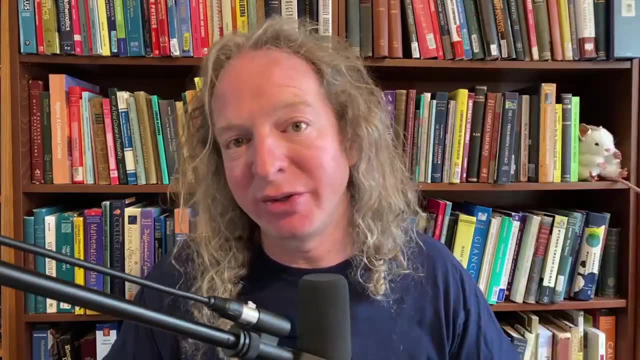 trying. It's hard to find really, really good books on partial differential equations. Another one I have is the one by Evans. That one is a little bit better than this one, So I'll leave links in the description. So that's one piece of advice I have is get some books on partial 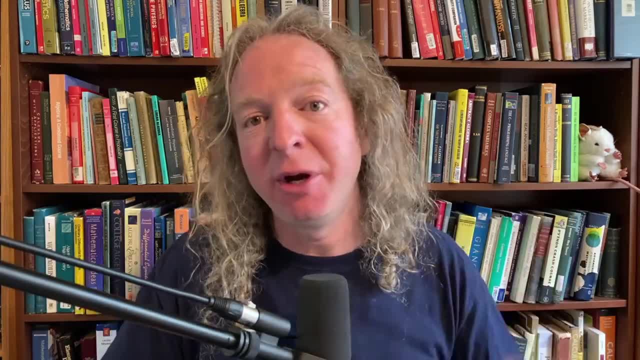 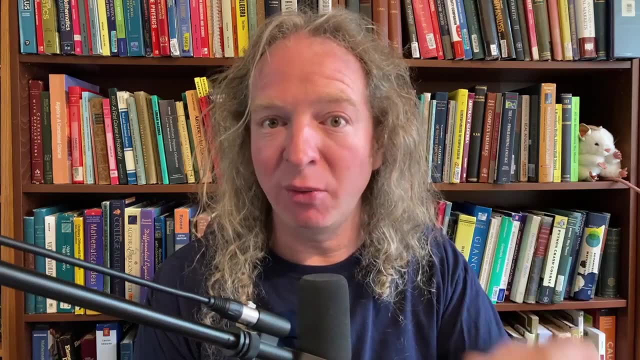 differential equations, And I say books plural. I'll try to leave a few that I have in the description, But beyond that I think there's more that you really should be doing when you're trying to learn partial differential equations, And by that I mean I really think it's helpful to take. 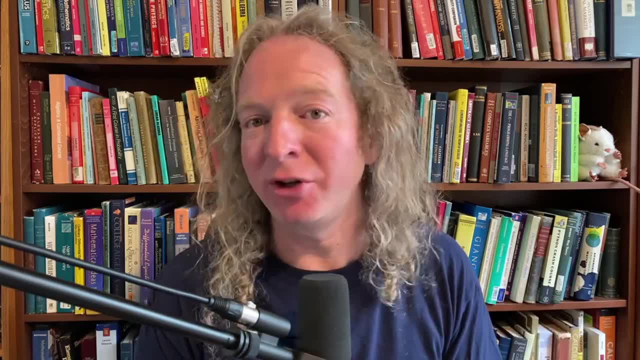 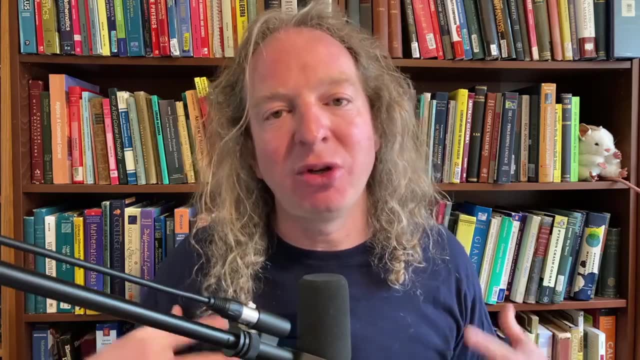 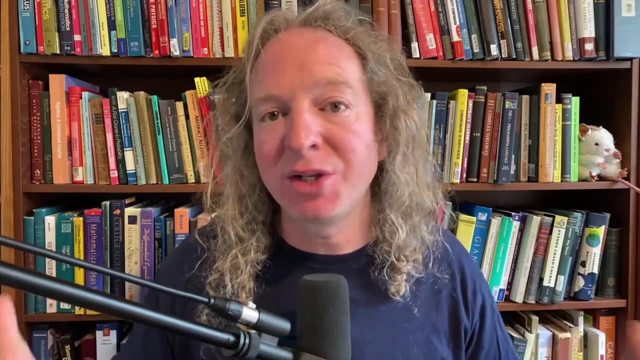 a class, It really helps. Okay, you can learn it on your own, Self-study is great, But PDEs, I just feel like having an actual classroom where you can go take classes is totally worth it. So if you're in the vicinity of a major university or a big college, usually they have a partial 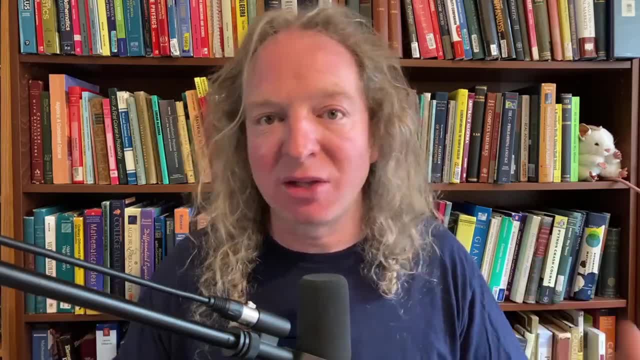 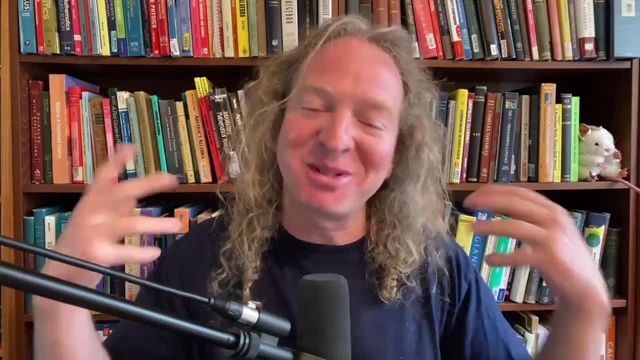 differential equations class And usually you can take it as long as you meet the prerequisites. If you don't, you can always go beg for permission. Please let me in. Sometimes they'll say yes. A lot of times they have really strict rules about that. They have this viewpoint where well, 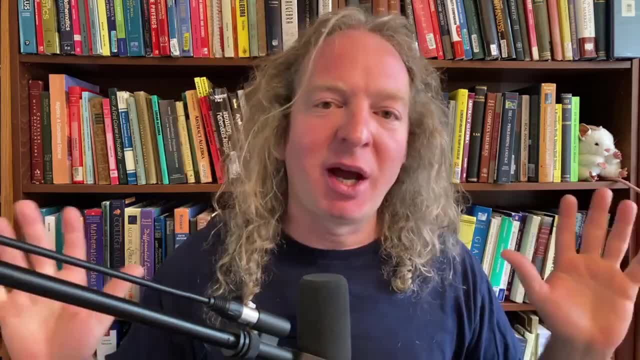 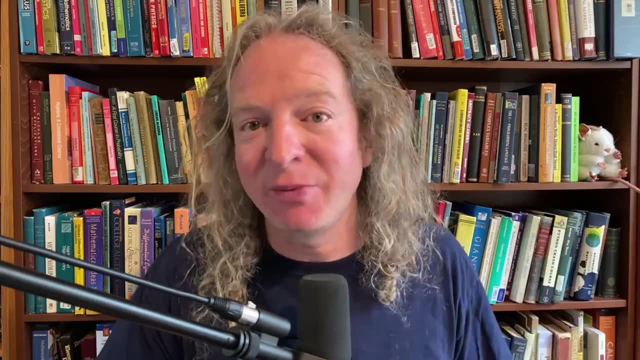 we're not ready for this class, so we can't let you take this class, which I don't know. if I agree with that viewpoint, I think that it should be open to everyone, But just realize that it's a tough class. You do need some calculus to learn partial differential. 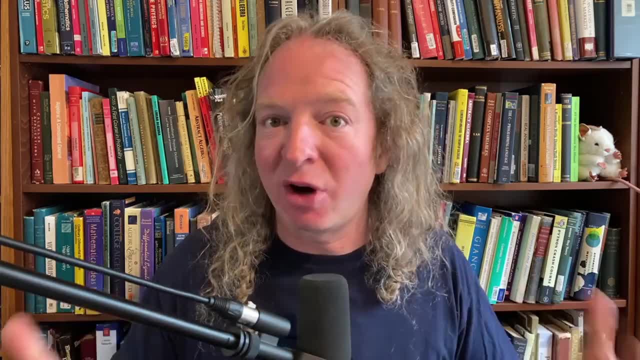 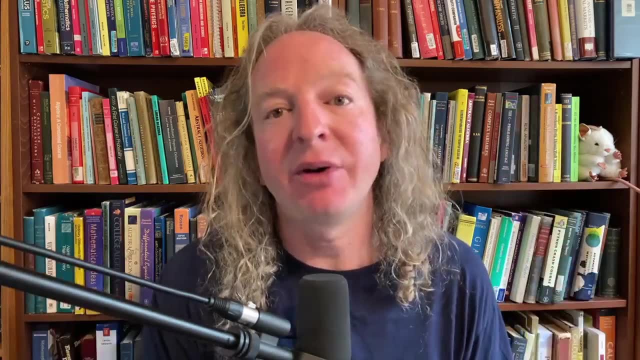 equations. In particular, you want to know what partial derivatives are. You want to have some multivariable calculus behind you. You want to have a solid class in calculus three where you're aware of all of those multivariable constructs that come up in multivariable calculus. You want 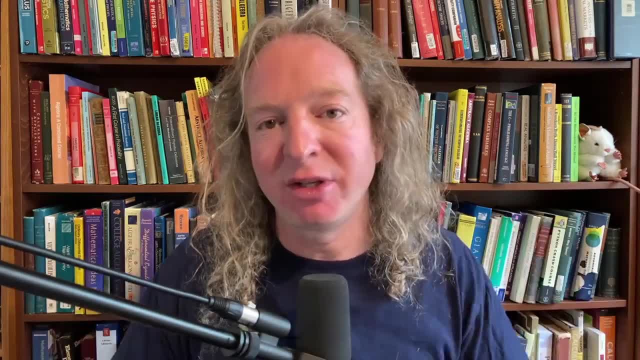 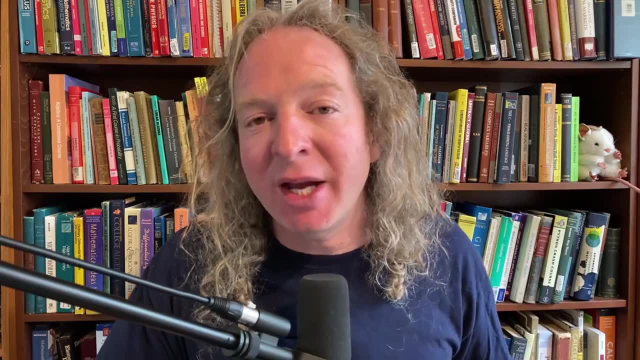 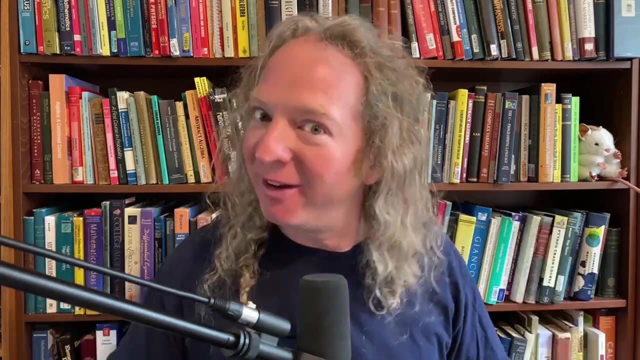 to know what the gradient is. You want to know what a directional derivative is. You also want to have a really strong background on ODEs, which is ordinary differential equations, And I emphasize that because my personal experience in partial differential equations I found that I was really using a lot of the stuff I learned. 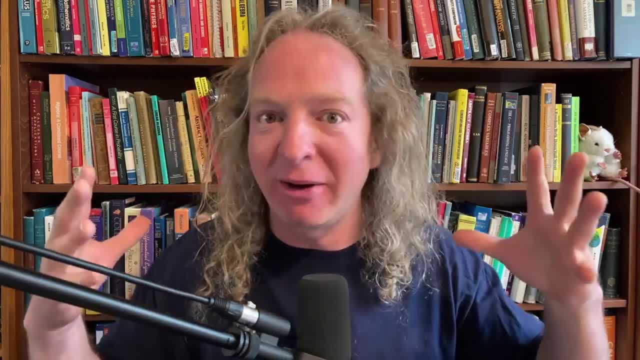 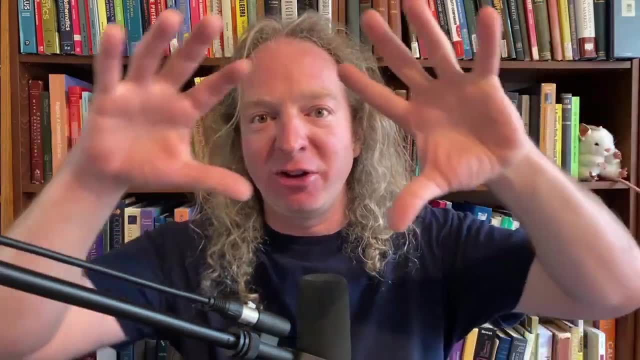 from my ODE class. I'm getting goosebumps now thinking about it, But it was really quite enlightening, because you're in this class, PDEs, and all of a sudden you have this equation and you do some type of transformation and you turn it into an ODE. 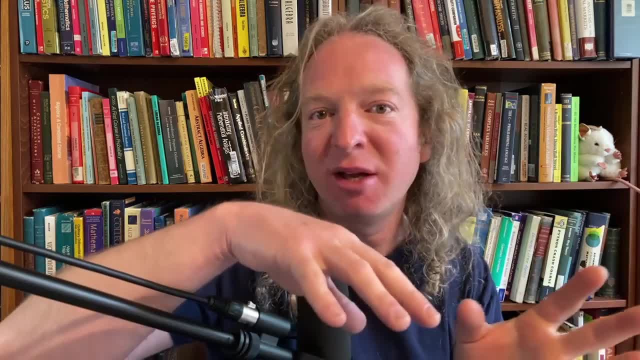 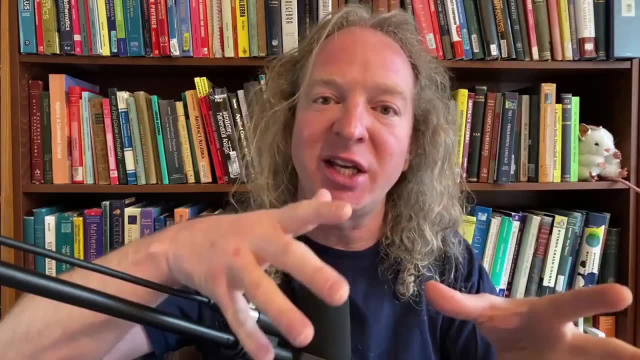 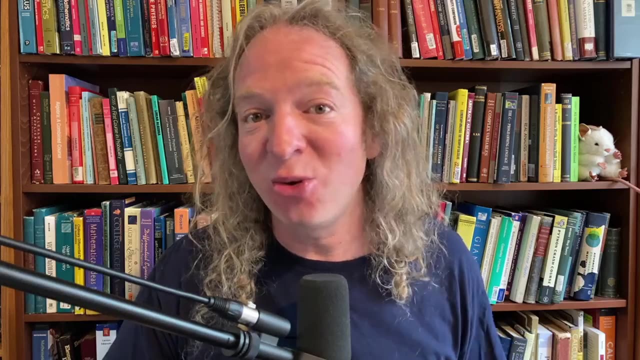 And then you use some technique you learned in ODEs, such as undetermined coefficients or variation of parameters. You use a regular differential equations technique to solve a partial differential equation And I think that makes it really really cool. So PDEs is a cool class. It's a cool subject because you use those old skills At the same. 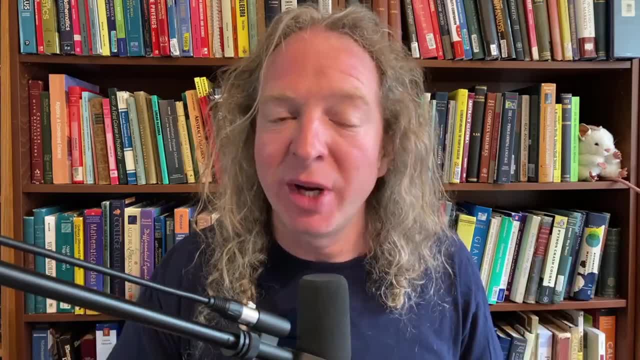 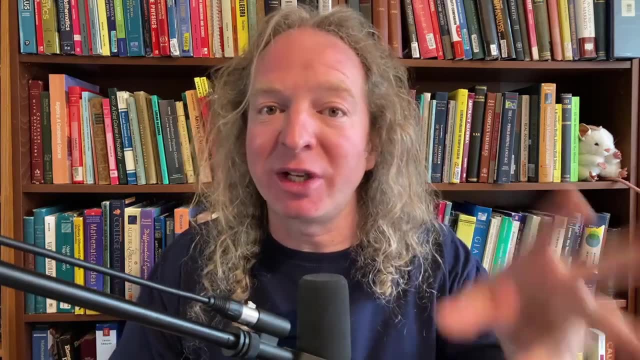 time. if you don't have those old skills, it makes it harder to learn. So it's a big learning curve for PDE And that's why I'm suggesting you take a course, because you're going to find that when you start studying PDEs you're going to say: 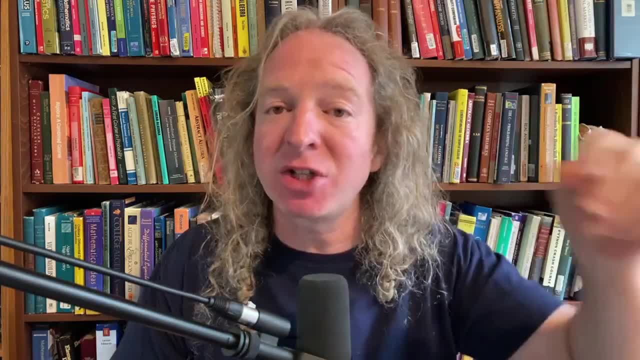 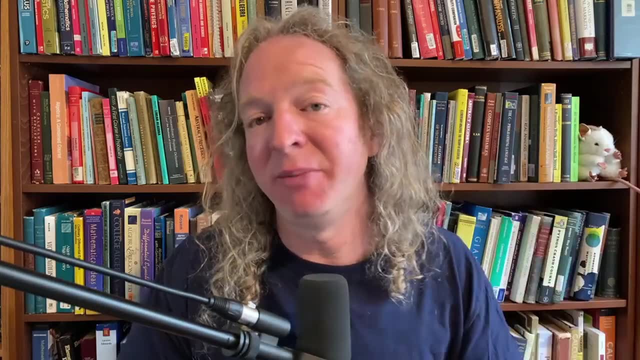 hey wait, what's that? And you're going to have to do a lot of backtracking, especially if you don't know ODEs and especially if you don't know some of the multivariable calculus constructs that come up in Calc 3.. So my advice is: get a couple of books Again. 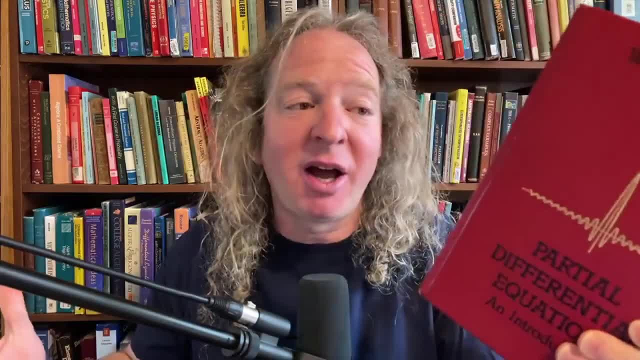 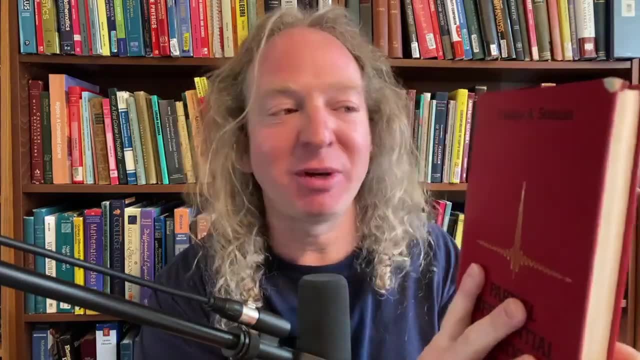 this is the one that I used for the course. I think it's pretty good. I like it. I like the color. I remember I had my friend once he came over and we sat out on the back porch and we were doing math.